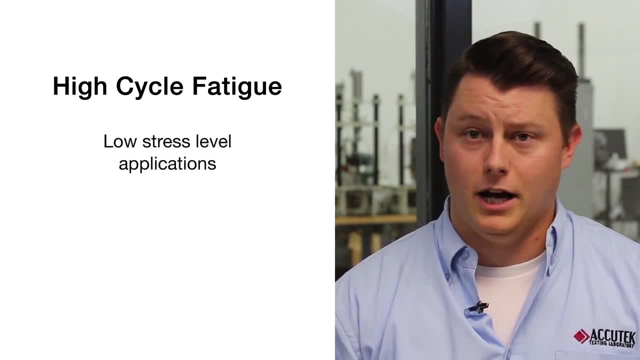 that experience stress levels that are relatively low. How does low cycle fatigue test work? Low cycle fatigue tests are used for materials that experience stress levels that are relatively low and where, at deformation, a change in shape or size of an object as a result of 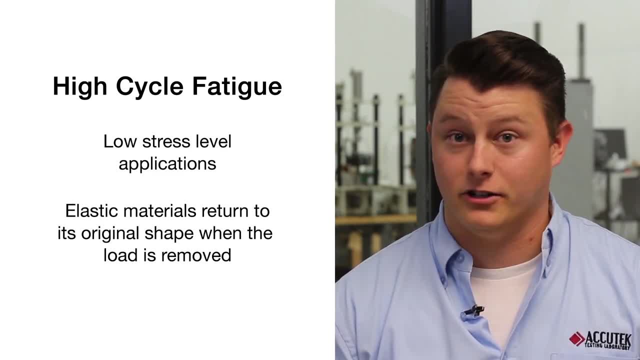 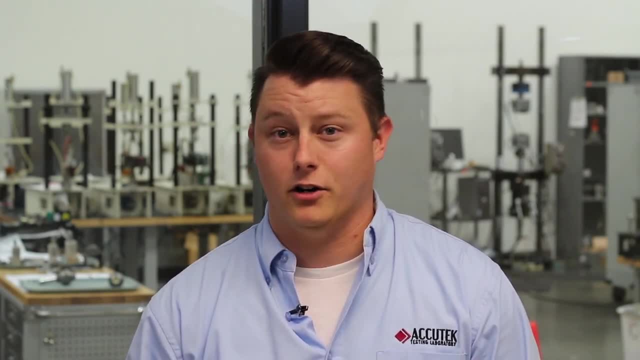 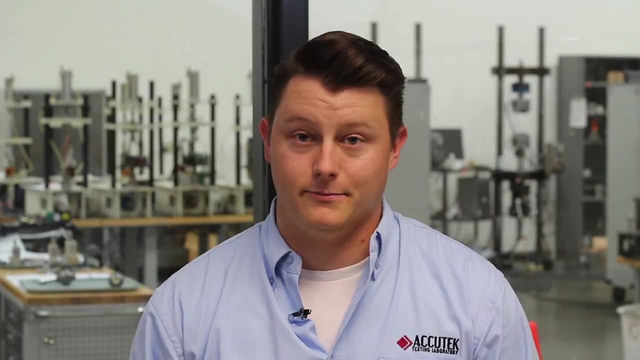 an applied force is primarily elastic in nature. The principal distinction between high cycle fatigue and low cycle fatigue is the region of the stress-strain curve where the repetitive application of load and resultant deformation or strain is taking place Due to material behavior. at low stresses versus high stresses, both methods are performed. 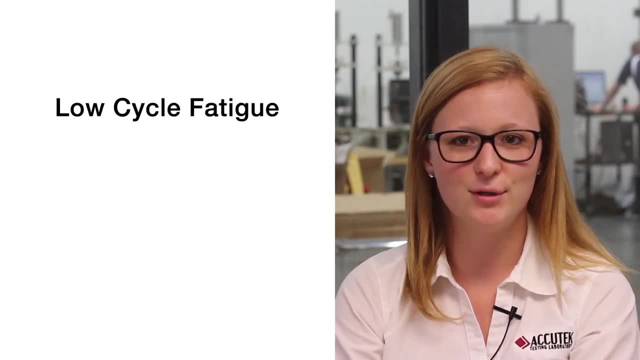 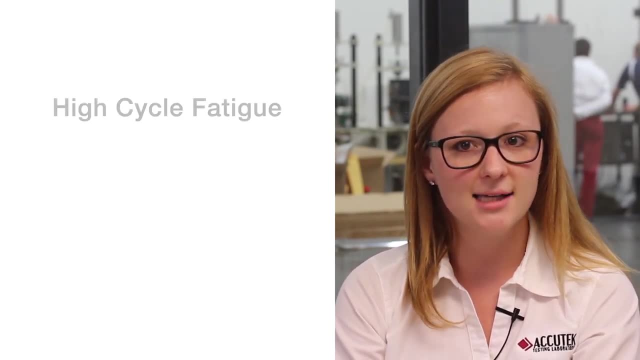 using different control methods. Low cycle fatigue is performed using the strain control method, where a specific magnitude of strain is applied to the test specimen per cycle. Traditional high cycle fatigue is stress controlled, meaning a constant load is applied throughout the duration of the test. 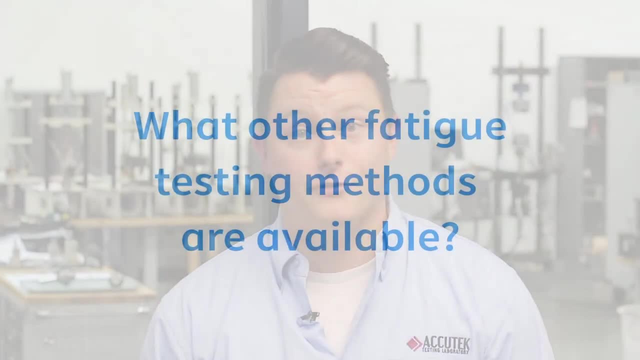 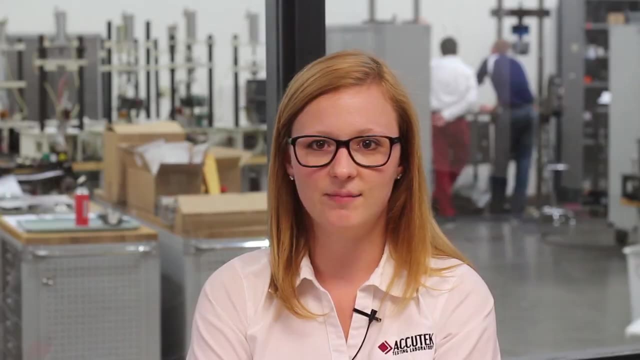 This leads us to our second most commonly asked question: what other fatigue testing methods are available? The most common type of cyclic loading a specimen can be subjected to is axial. This is where the test specimen is taken from tension to compression repeatedly. The most common type of cyclic loading a specimen can be subjected to is axial. This is where the test specimen is taken from tension to compression repeatedly. The most common type of cyclic loading a specimen can be subjected to is axial. This is where the test specimen is taken from tension to compression repeatedly. The most common type of cyclic loading a specimen can be subjected to is axial. This is where 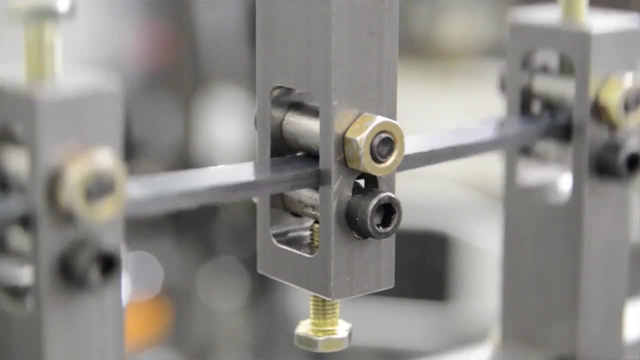 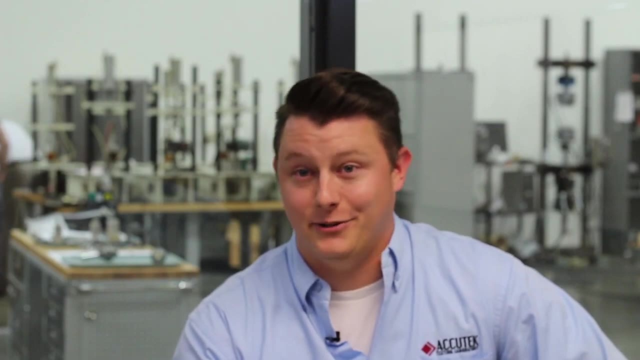 the test, specimen is taken from tension to compression repeatedly. In addition to the traditional axial, high cycle and low cycle fatigue, flexural or torsional stresses may be applied repeatedly until point of failure. In general, axial is the most popular method for traditional fatigue studies, Rotating. 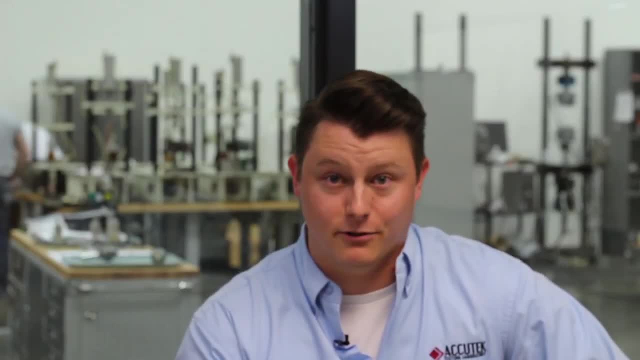 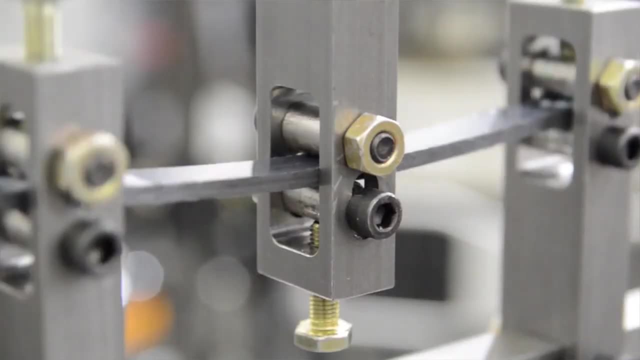 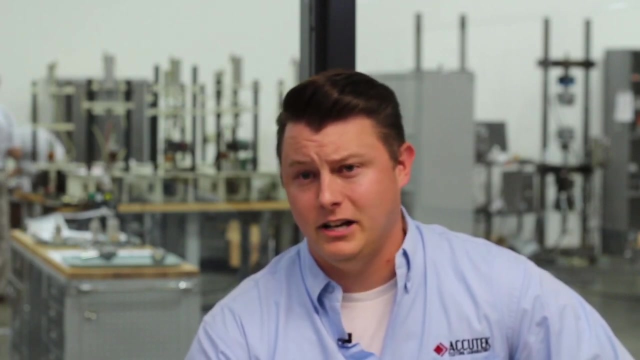 beam is also a very useful method for generating high cycle fatigue runs in short intervals of time. Torsional, sheer and flexural methods are mainly geared toward materials that are susceptible to specific stresses. a material expected to see high concentrations of oscillating torques, for example, would most likely benefit. 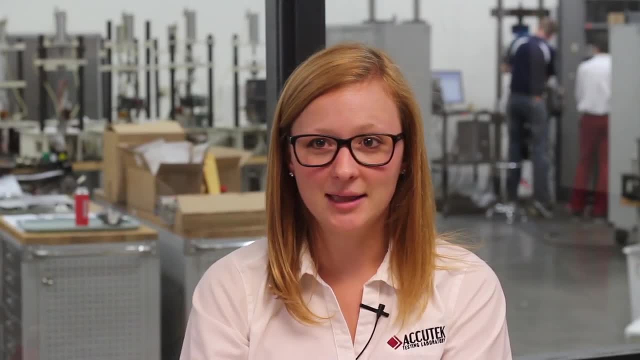 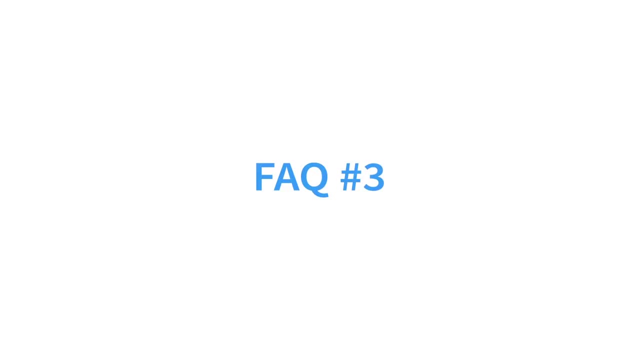 from a torsional fatigue study. thanks, Kevin. also keep in mind that by carefully studying your material application, you can determine which method will give you the most relevant and useful results. what is an R ratio in fatigue testing? simply put, the R ratio is representative of the loading profile.